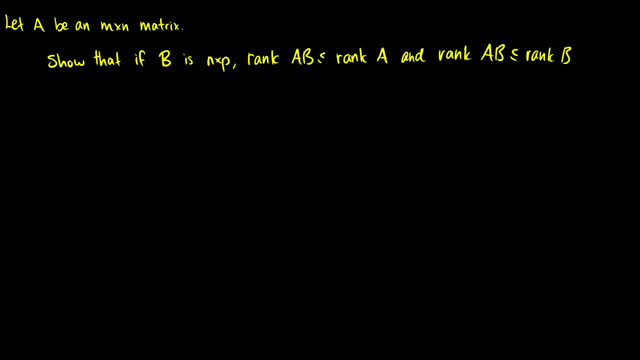 This video we're going to do a proof with ranks. So let A be an m by n matrix. We want to show that if a matrix B is n by p, then the rank of A, B is less than or equal to the rank of A and the rank. 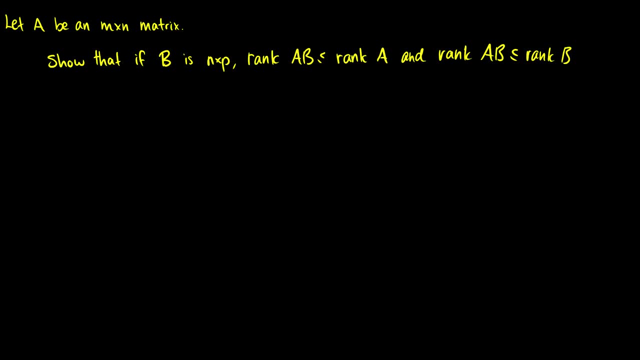 of A. B is also less than or equal to the rank of B. So there's really two questions here. A will be rank A. B is less than or equal to rank A, and then B will be rank A: B is less than or equal to. 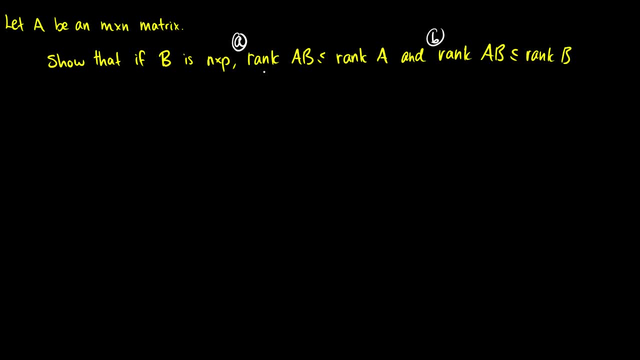 rank B. Okay. so the first thing is we should remember that the rank is really just the dimension of the column space. So when we say rank A- B is less than or equal to rank A, we're saying that the dimension of the column space A- B is less than or equal to the dimension of the column space. 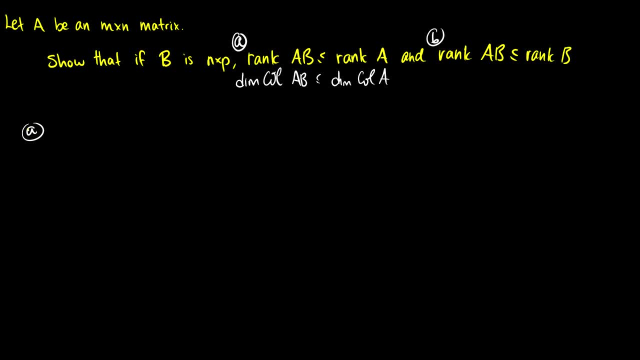 of A. So for part A we're going to start by taking a vector V and it's going to be in the column space of A- B. So what this means is that we can write any vector V as A B times some other vector X, Using the 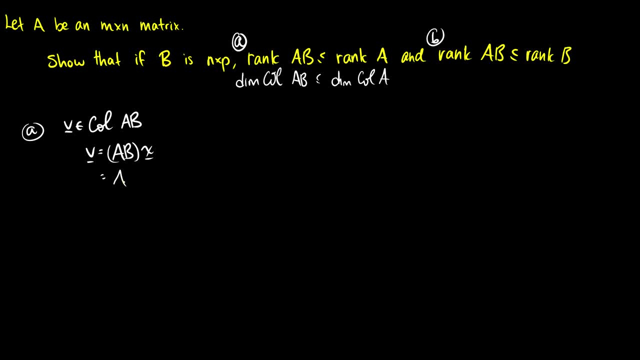 associativity properties. we could also write this as the matrix A times vectors B, X. So what this means is that this vector V is really just a linear combination of the columns of A, So we can say that V is less than or equal to the column space of A. So we can say that V is less than or equal to. 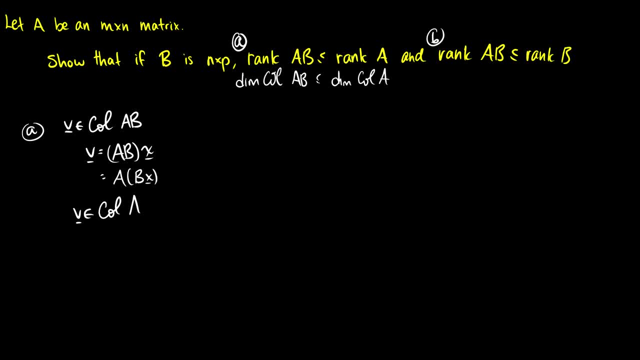